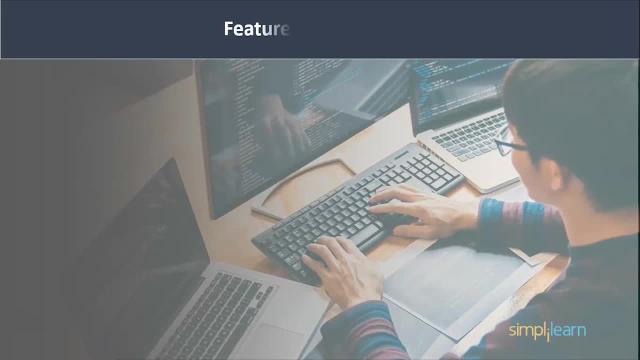 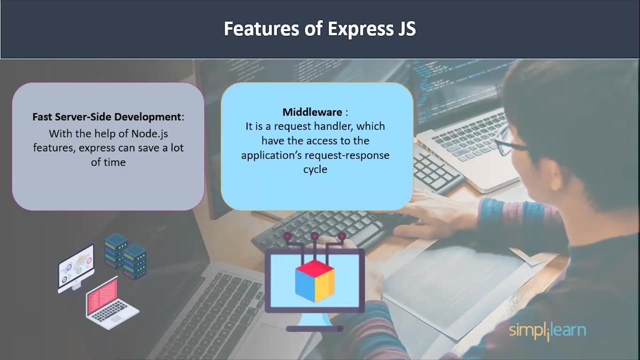 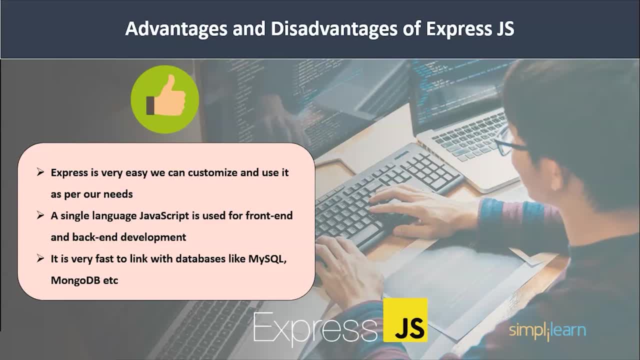 fast, lightweight and easy to use. ExpressJS is a very high performance: fast, lightweight, MongoDB, etc. Let's see the disadvantages. The disadvantage of ExpressJS is that there is no structural way to organize things. Sometimes the code becomes non-understandable.